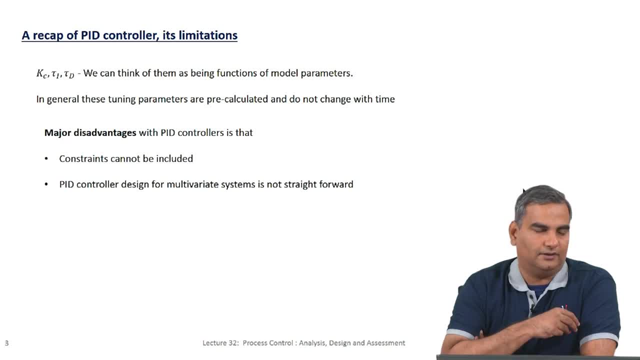 is going to be KC times error. Now, that is basically saying I see this error, I am going to make this change and if you are also going to look at past errors, then you are going to do an integral EDT. and if you are going to also look at future, then you are going. 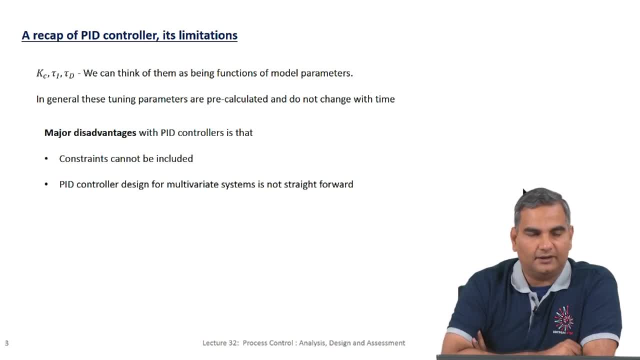 to do DE by DT, and the parameters that multiply the integral at term and the differential terms 1 over tau I and tau D. Now, clearly, depending on what process is being controlled, these parameters are going to take different values, So in some sense you can think of these parameters themselves as being functions of model parameters. 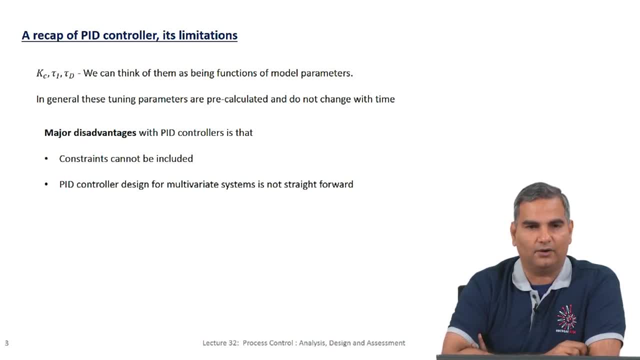 So you might actually say: look, PID is also using the model in some form to come up with these parameters: KC, tau I and tau D. Nonetheless- we have been discussing this for a while in this course- these tuning parameters are pre-calculated and they do not change with time. generally, 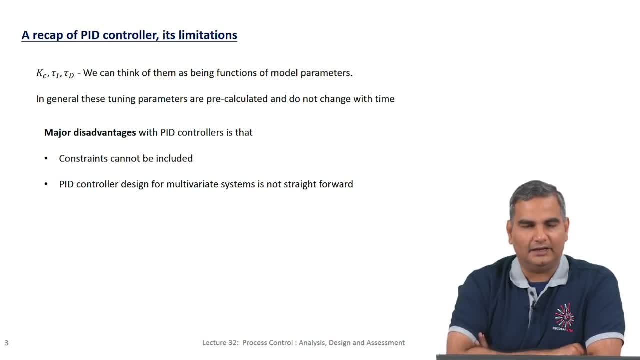 there are also gain scheduling, There are individual PID controllers and so on, but in general, as far as we are concerned in this course, these do not change, and while these parameters are actually computed as different numbers for different models, they still only encapsulate some notion of the 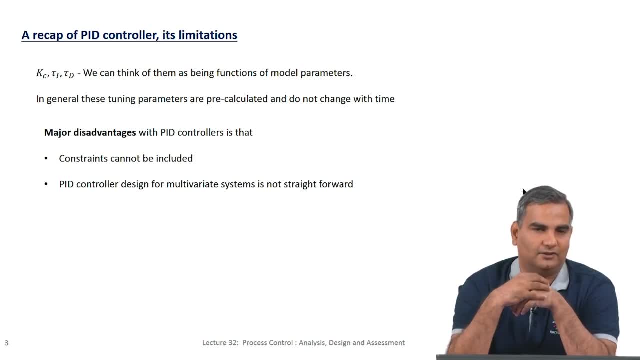 model. those are not directly model parameters themselves. So that is something that we have to keep in mind. So we saw that as we wanted to control more difficult systems, then we had to go away a little bit from the PID framework, most notably for the time- delay control- where we had to really use the model already in the 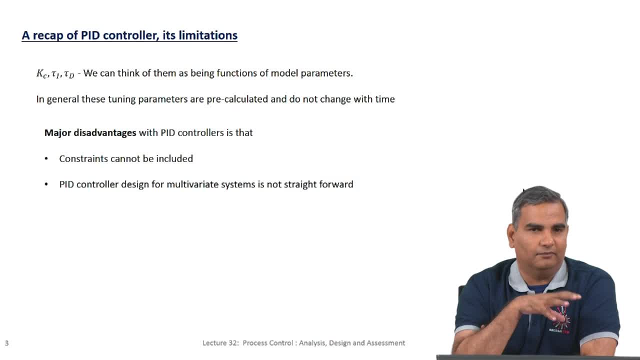 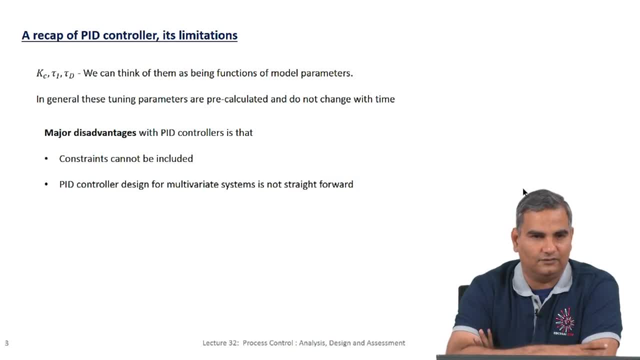 the control loops are still PID loops because they are very, very effective, very simple to understand and very simple to tune and work with and so on. But there are problems which require little more sophistication and that is where we start talking about model predictive controller and other types of controllers, and we also 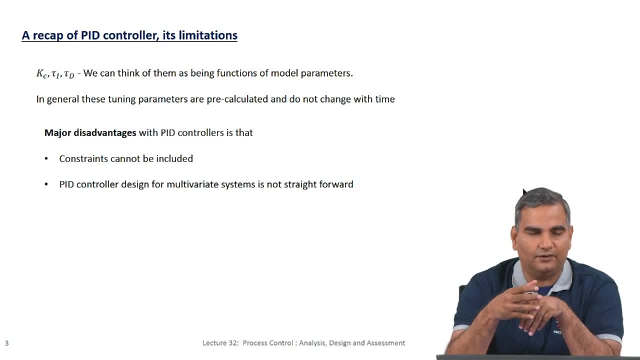 noticed. actually, for processes with difficult dynamics, such as, let us say, inverse response process, We saw that we still came up with a PID controller only and if you take the example of the time delay system, we still came up with a PID structure only, except that the error was also. 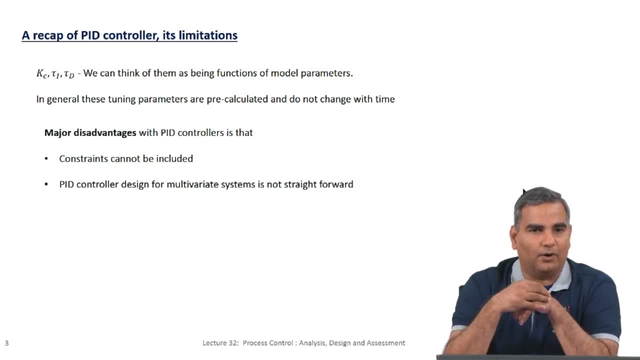 including another term- which was calculated from a model. but still, once this error was modified by using some of the model computations, also that on that modified error we still had a PID controller working. So in some sense PID controller is a very powerful idea that that is really useful, and in fact for unstable systems also, if you. 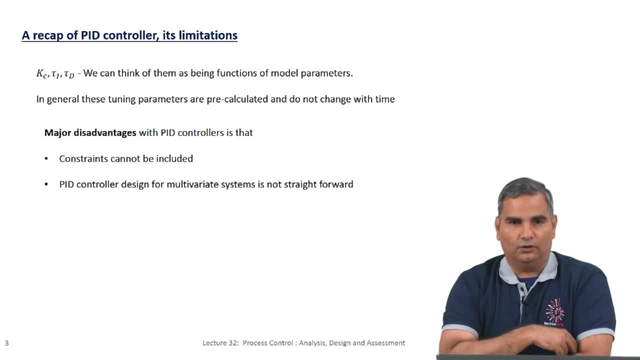 remember we came up with a PID controller, right? So basic loops are still PID controllers. if there are difficult dynamics, then there are PID. there are things that you do to modify the PID controller to make it work better. Same with cascade control. cascade control again. you will have two controllers, one P. 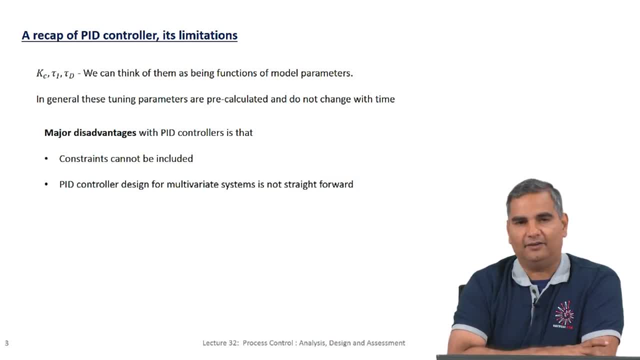 and maybe outside. PI controller and feed forward controller is basically a PID controller, PID again going to be a PI or PID controller with some input from the model for the disturbance. okay, So in that sense, even the difficult dynamics you can think of as modifying the PID controllers. 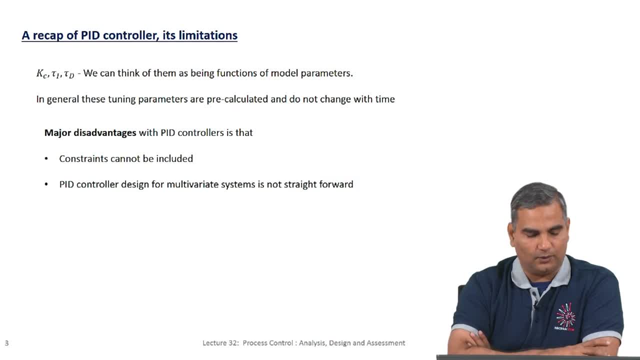 with more structure, or more model information and so on. However, if you really want to address this as a multivariable control problem, then either you have to do some kind of decoupling, which can become complicated after a while, because the more decoupling you do, based on 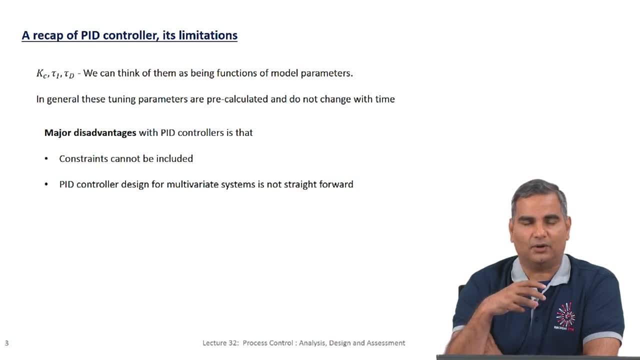 this model, then the one has to worry about how certain this models are, what happens to the uncertainties, and so on. So in general one could assume that PID controller design for multivariable systems is not straight forward. so you have to really be careful about how you design these controllers And 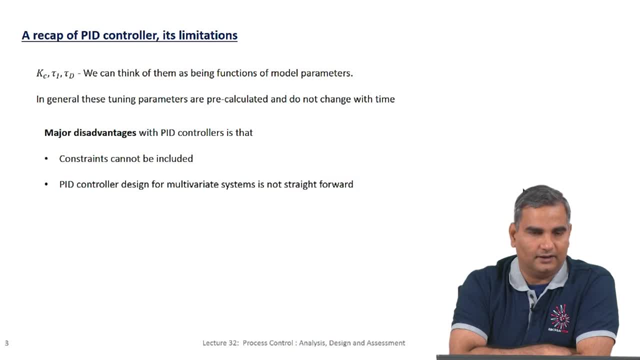 other big disadvantage of PID controllers is that we cannot include constraints in the control. okay, So this is the first time I am using this word constraints, so I want to explain what this means. So when we do this- computations with PID controller- we compute U as some function of error and 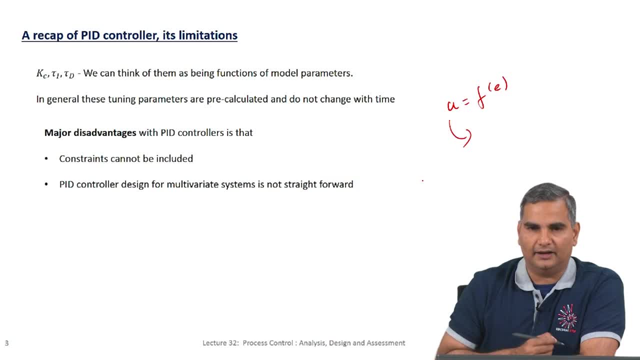 whatever value we have for U, we assume that the manipulated variable can take. So we never think about what is the maximum value U can take. And this is because, after a while, though we try to connect the physical system with control and so on, after a while we start getting very accustomed to looking at these variables. 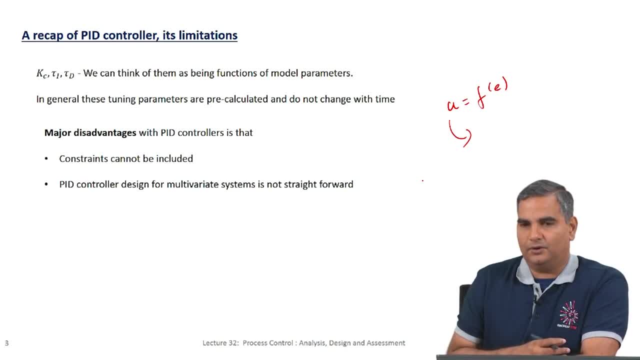 and then say Things work alright, But really think about flow control. you have, letís say, input, feed, flow of water. now, based on the pipe dimensions and based on your control valve, there are going to be various constraints Based on the pipe dimension and the pressures that 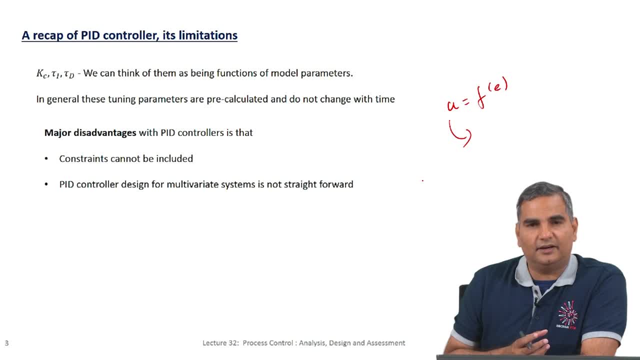 the pipe can withstand and so on, there is definitely going to be a maximum flow that you can get. So basically, the U itself is going to have some upper bound value, right? So if it is flow, So you cannot have more than this flow in a pipe. This is something that we intuitively 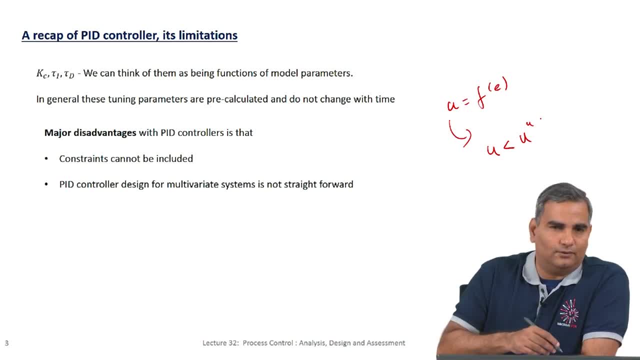 understand, But this is never factored into the PID controller. One way to factor this is to say, if the PID controller computes an U which is much greater than the maximum value this U can take, basically just keep it maximum value open, right, and then donít do anything. 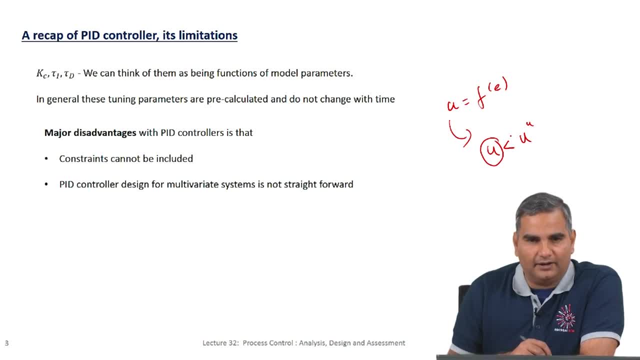 Now, this is what is called clipping in PID control. However, this can create all kinds of problems Which we will see later, So it is actually better to explicitly include this constraint in the controller design rather than saying: let me compute controller value for U and. 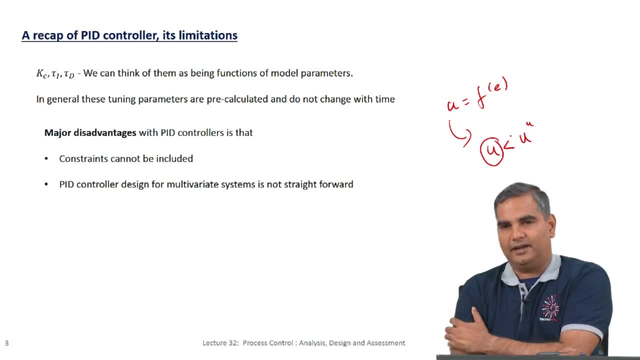 then basically decide whether that value can be taken or we need to clip that value, and so on. So that is something that could be handled better, more explicitly. So this is one. The other thing is, when we talk about controllers, when we talk about letís say, 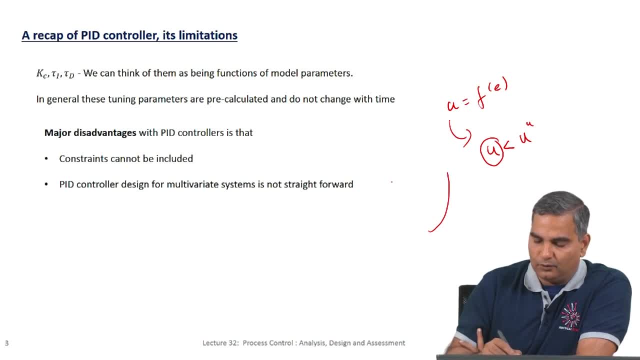 I have a U profile like this. So basically, itís not only the upper limit on U- okay, that is of importance- Itís also rate of change of U. So what does rate of change of U mean? Supposing, letís say, you think about a standard pipe that you use. So you kind. 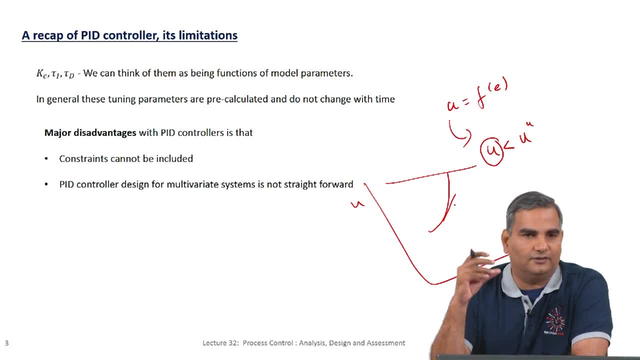 of open and close the tap right Now. if I ask you to get the tap to be completely closed and completely open the next second right Now, think about this. Supposing you had to really open the tap, you might not be able to do that in a second right. So the rate? 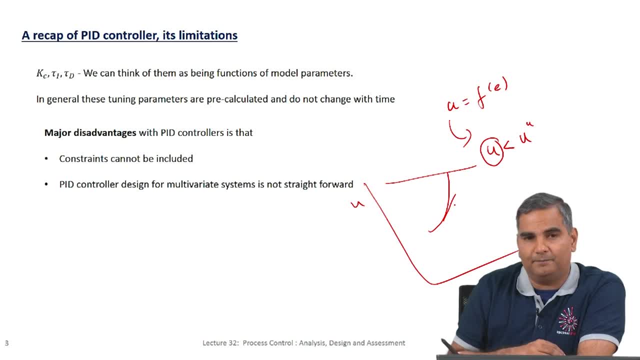 at which you can change the U is also limited. okay, So a completely closed pipe. if you want to open the tap, to fully open, if you are physically doing it, you know, depending on how many rotations you need to do, and so on, it might take you 5 seconds, 10 seconds, whatever. 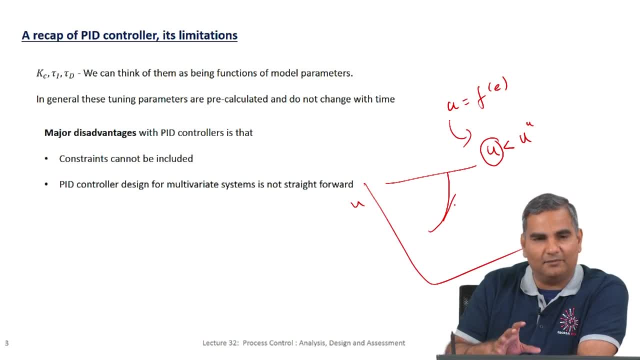 it is, Whereas the PID controller in its computation is not taking this into account at all. Itís just saying the U is this and then the U profile. Lecture 1 of 9 Profile is this: That basically says D U by D T can get to values that are not feasible. 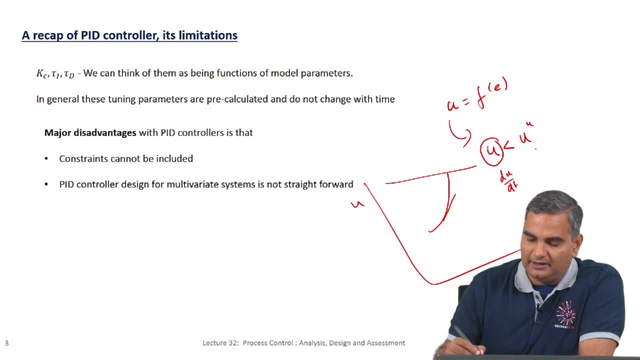 in real time. So there is also a constraint on D? U by D T, or Iím going to call it delta U, because we are going to move on to a discrete formulation quickly, So this will also be constrained. So within a short period of time I can only change U by this. much, right, That? 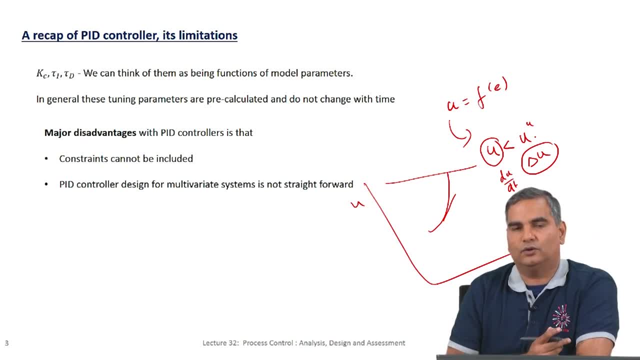 constraint is never included in PID design. So this notion of you know constraints, you know constraints for the manipulated inputs and how you include them in a controller is a very important question and, of course, PID controller was never designed originally to take this into account. 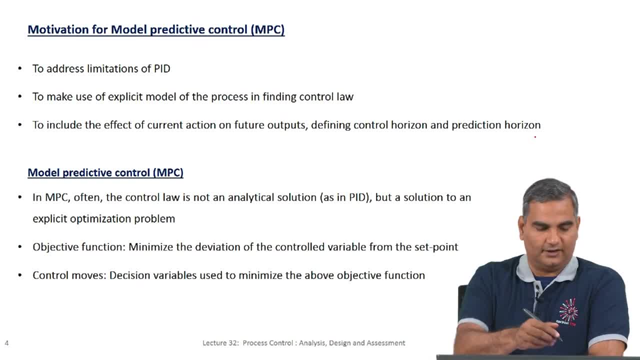 So the idea of model predictive control is first to address the limitations of PID. the basic limitations of PID are: constraints cannot be used, and number 2 is that when multivariable controls the constraints cannot be used, and number 2 is that when multivariable controls 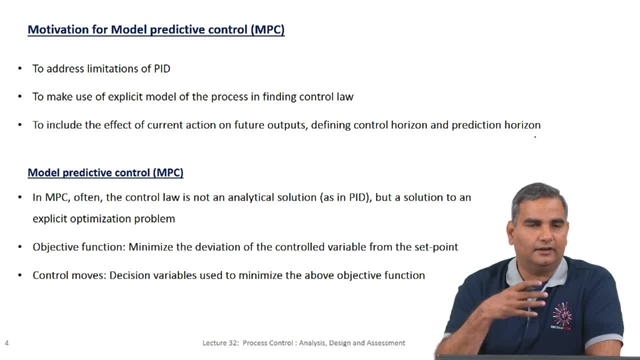 the constraints cannot be used. So this will be the first point. The second point is that variable processes are there, the deriving this, PID controllers become more complicated. So model predictive control you can think of as being thought of to address these limitations. 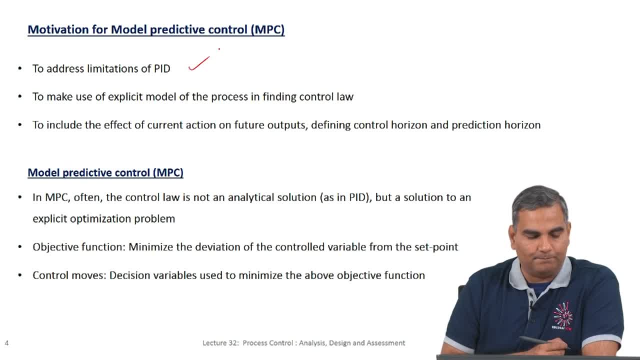 Now, model predictive controller is also going to explicitly use a model of the process and finding the controller. now, as I mentioned before, in a typical PID controller- though, we can think of this KC, TAUD and TAUI as being derived from the model parameters- they 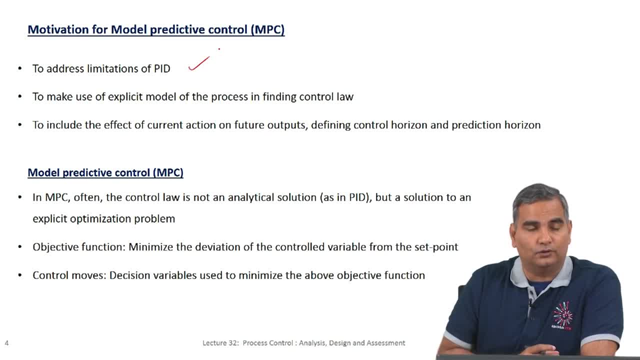 are not model parameters themselves, they are not the model themselves. So explicitly a model is not being used in finding a controller, whereas in model predictive control we will use the model of the process directly in finding the controller. And then in model predictive control we are going to start introducing the notion of horizon. 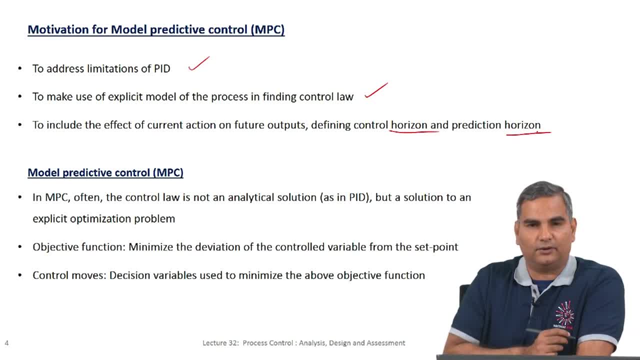 okay, There is going to be controller horizon prediction. We have never talked about this till now. I just will allude to this here- and this is going to be a key difference between PID and model predictive control. So in simple layman terms, to explain this now, if I am looking at output for a PID control, 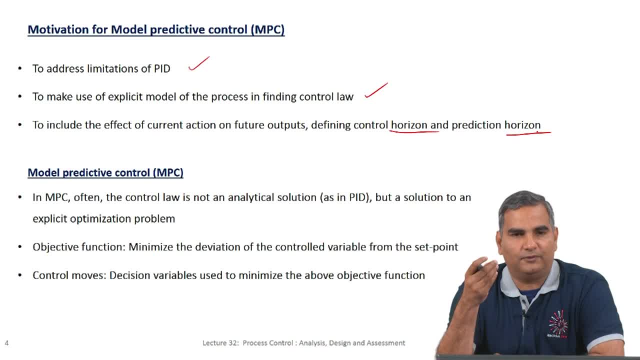 at a particular time. I am looking at the difference between that output and a set point at that time and I call that as error And all the decisions that I make are based on the PID control. It is based on the current error right. if it is a K or in other cases it might be based. 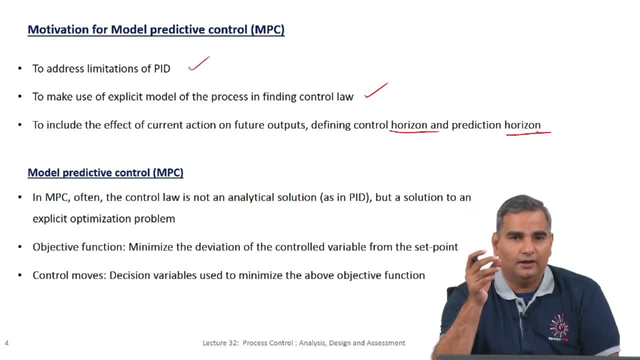 on my past errors. it is based on if you do DE by DT. it is based on the rate. but you can think of if you do a backward difference. you can think of the change in the output between the last time and the current time. 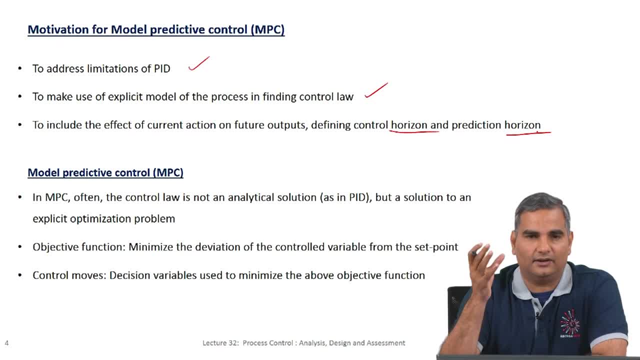 So, in other words, everything is based on whatever errors that we have seen and the current output and how far away from the set point, Whereas we might actually think about not only the error now, but what is the error likely to be in the future if I make a control move currently right. 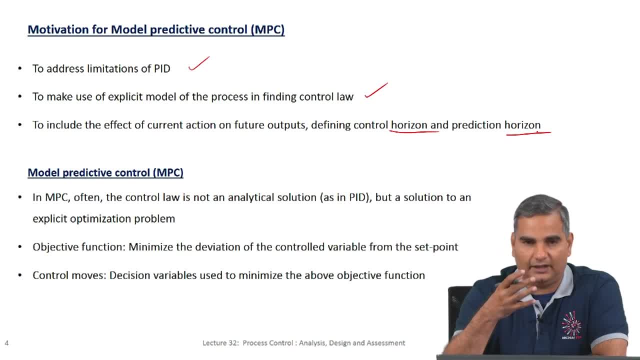 So that notion of a horizon into the future that we can think about from a control viewpoint. So this is something that we always do in our life. Basically, no decision is taken only based on all that has happened before and what you have currently. We always take decisions based on the current output. 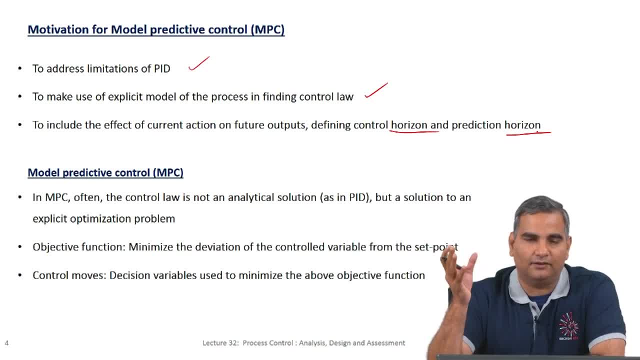 So this is something that we always do in our life. It is based on what we think is an optimal thing for us to achieve. So you might have heard this in most interviews. they will ask you: where do you want to be 5 years down the line? or one might ask: what skills do I want to get in the next 3, 4 years? 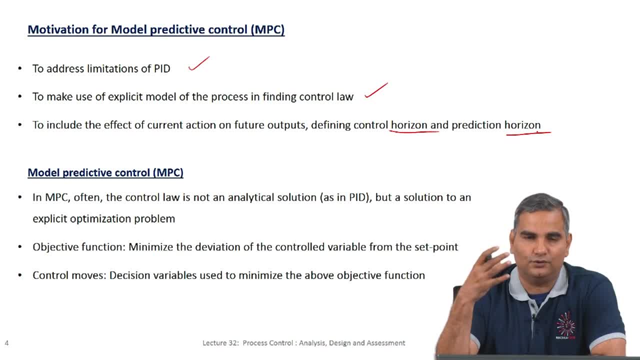 So all of this have a notion of horizon into future. and it is not only okay. I want to improve myself today, right? So if you want to learn, let us say musical instrument, you cannot say I want to learn it today. You know where will I be with this instrument 3 years down the line, 4 years down the line. 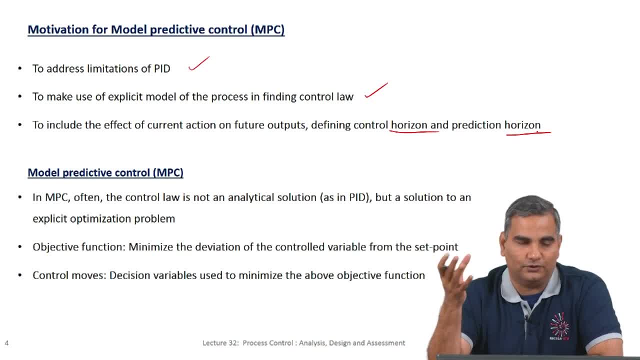 and so on. So that is the kind of future outputs in terms of performance matrix that we want to decide right, And how do I include that in a controller design? that can be done using model predictive controller, using this notion of horizon, which we will see, okay. 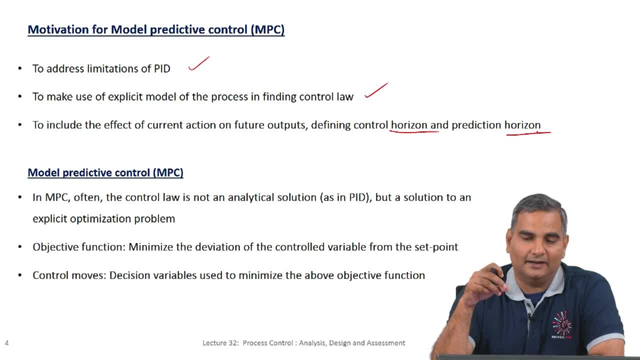 So now, another very interesting thing is that so, since we kind of restrict ourselves to looking at the error currently and the past error, and maybe just one error next error or one before, when we do the derivative term, Basically the control action that we are planning for is only at the current time right. 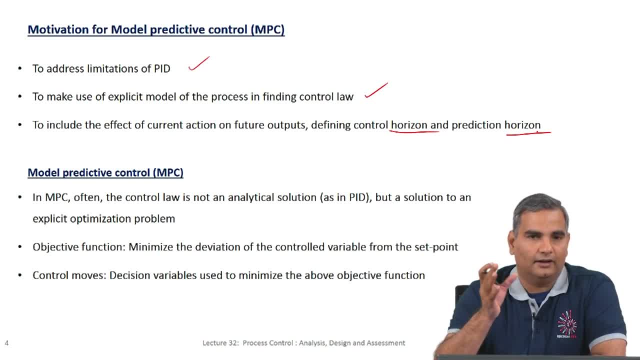 So we only get a current control move, u. okay, Now error is based on past and d by dt and e, but the control move is only based on u. But again, think about how we will 1.. 1. think about how we will look at this in real life. 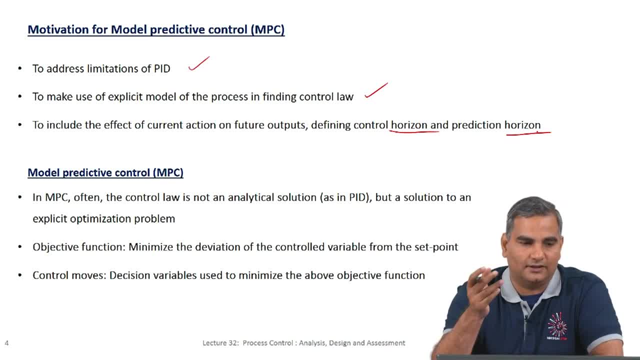 Supposing you said I told you this interview question right. So they say: where will you be 5 years down the line? If you said 5 years down the line I will be so and so, then in your mind there is always this question of if I have to be so and so in 5 years, then I have to do these things. 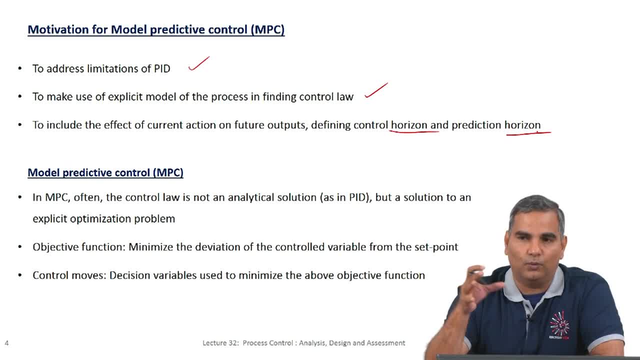 in the next year, these things in the year after that, and so on. So while you set yourself targets for a certain number of years, years, and say this is what I want to achieve, the effort that is needed to achieve that is also being planned at that current time itself. it is not as if I have to be so and 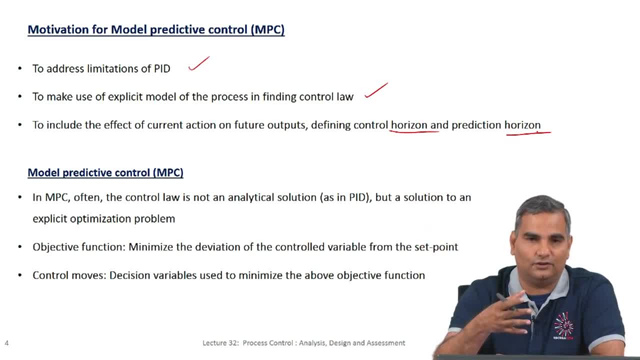 so for yesterday, I do this. that is not the decision you take, right. so you take: okay, I have to do this, I have to learn this, and so on. so you are also deciding about what you need to do at that current point and little bit into the future so that you can be so. 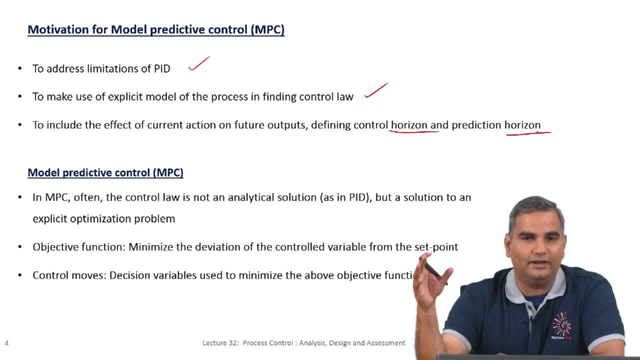 and so clearly you will not plan for what you should do 5 years after your time because your goal itself for a 5 year goal. so maybe you will say, look, if I have to be this in 5 years, at least the next 2,, 3 years, I have to do this, this and this. right, so you are. 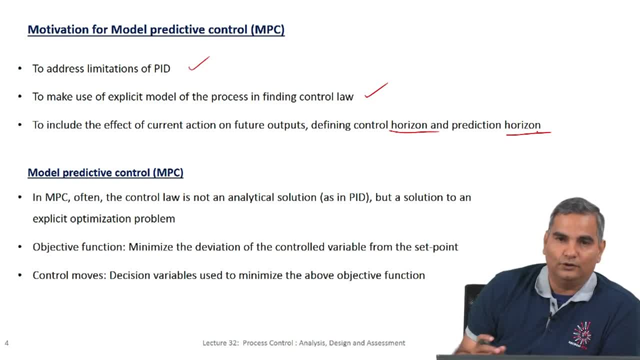 already planning for the next 2 to 3 years, so that again brings in a notion of horizon. so the control move: you are planning not only the current control move but you are also planning into the future. And based on these control moves into the future, what is the output that you are going to get and that 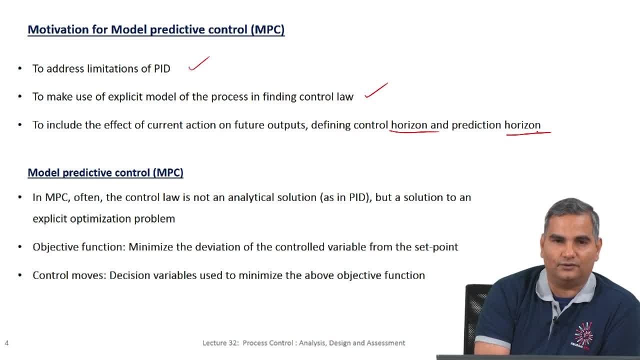 is also into the future. so all of that is this notion of horizon. so model predictive control enhances the framework of PID by looking at constraints, as we talked about in the last slide, looking at using the model explicitly in finding the controller, and then also this: 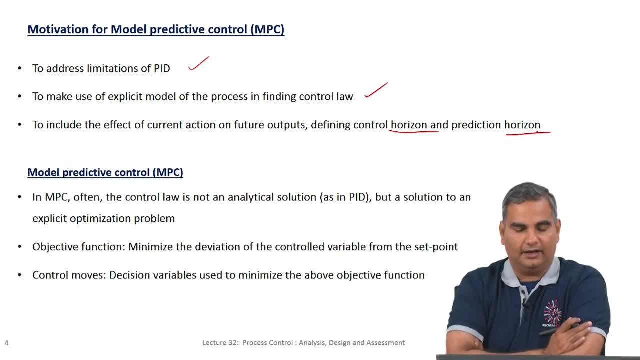 notion of horizon, which is what we will talk about, and then I will show you mathematically how this is done in model predictive control. Now, model predictive control basically solves an optimisation problem at every time, so this optimisation problem is solved and the solution to the optimisation problem itself. 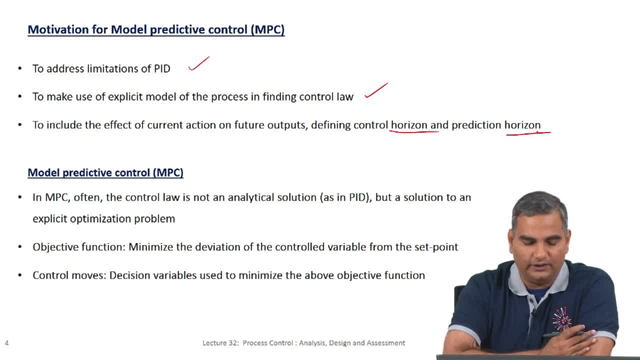 becomes the computation of control moves, or U. so in that sense it is not an analytical solution like a PID. right PID is basically, you will say K, KC, error plus 1 over tau, integral, EDT plus tau, D. So this is an analytical expression, whereas U in a model predictive controller is a solution. 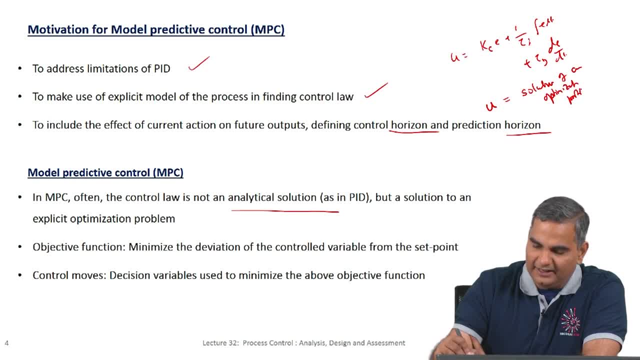 of an optimisation problem. okay, Now, in the linear case, people have shown that you can actually show that even in an optimisation solution you can get some analytical forms and a gain of that analytical form changes over period of time and so on. so those are more advanced concepts, but as far as we are, 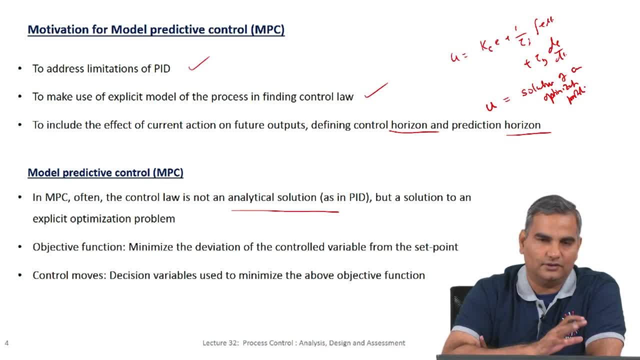 concerned in this undergraduate control class. you just need to know that it is a solution to an explicit optimization problem and not an analytical expression like this which is used in PID. The minute we talk about a solution to an optimization problem, we will describe this in little more detail in the next lectures- but when we talk about an optimization problem, 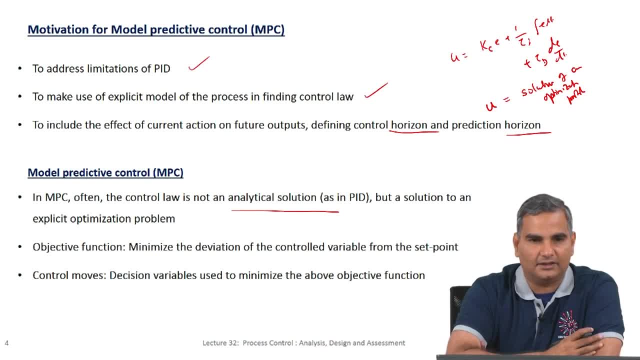 then immediately we have to talk about what is called an objective function, we have to talk about the constraints and we have to talk about decision variables that are used in the optimization formulation. So we will describe this in detail as we go forward. but the key difference that I just 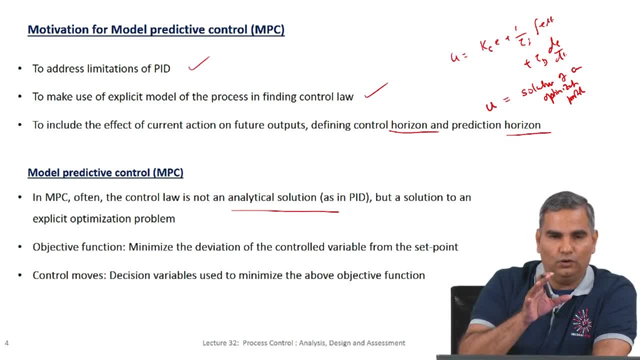 wanted to point out is that the U itself is computed as a solution to an optimization problem. So if I want to summarize this slide, then there are three main features of MPC which are different from PID. The first feature is that an explicit model is used at all times. okay, and now we have. 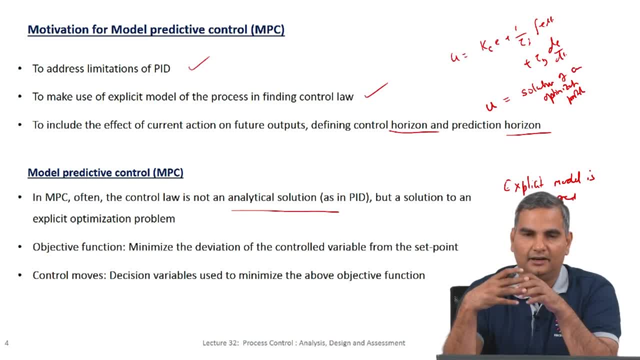 started with PID, which is an analytical expression. then we looked at as we kept learning more and more, started using more advanced concepts. we saw how a model starts creeping in within the PID framework. Now MPC is completely abandoning the PID framework and directly using the model in control. so 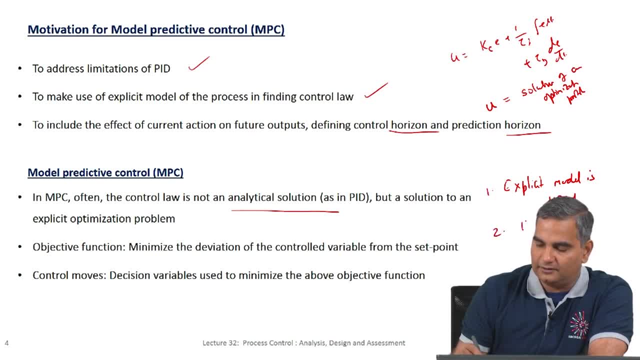 that is one big difference. The second difference is the notion of horizon, which is: I am not going to make plans for a control move only now, but I am also going to make plans for control moves into the future. that is something that we talked about. and the third important difference is that this: 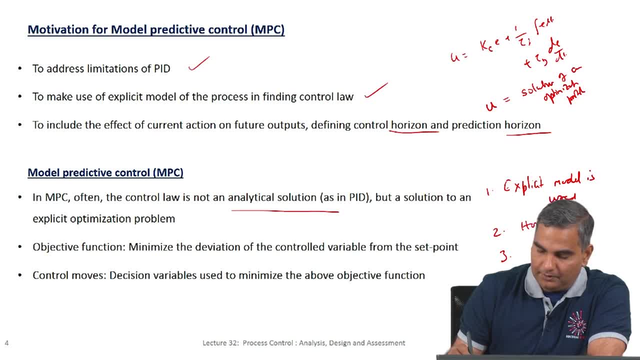 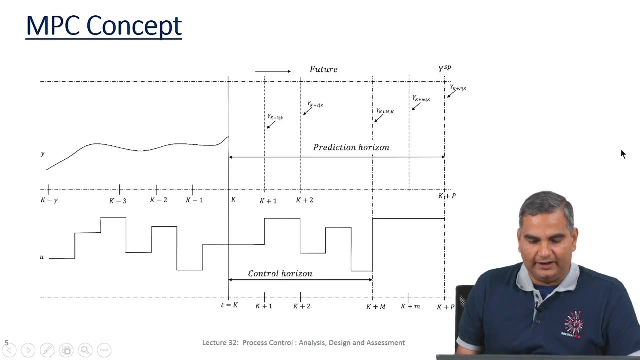 is going to be an optimization problem that is solved, which is solution to which is the control move, And it is not an analytical expression like what you see in a PID control. So we will look at the concept of MPC in more detail here. Now there is another change that we are going to introduce before we can formulate the MPC. 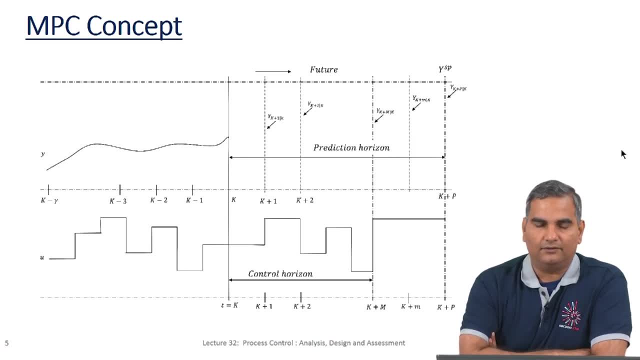 concept, which is basically till now, we have looked at all transfer functions and all variables as continuous variables, whereas we are going to start looking at this notion of discrete, Discrete variables when we talk about MPC control. I will explain that in good detail as we go forward. 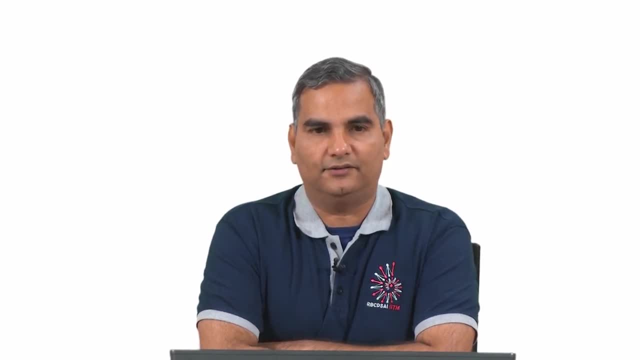 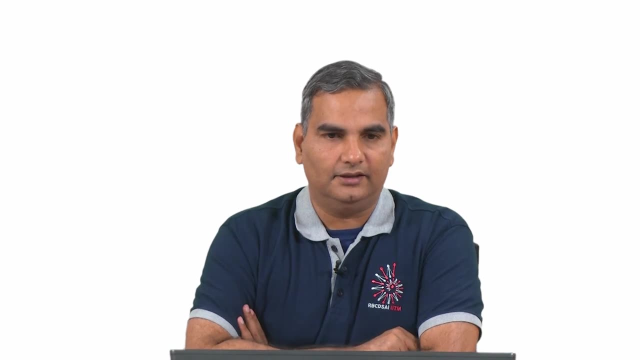 So now that I have kind of explained the differences between MPC and PID, I will come back to each of these ideas in more detail and show you how we can formulate MPC control for first- single input, single output Systems- and then show you how you can extend that very easily to multivariable systems.